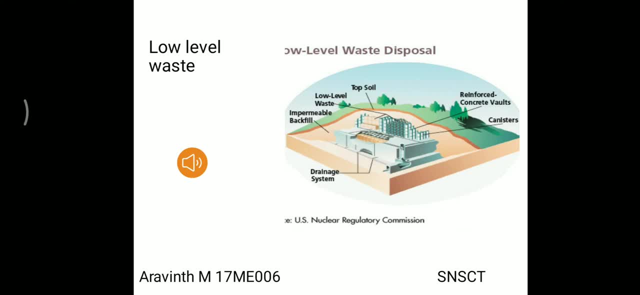 small relative to other thermoelectricity generating technologies that we use so far. Used nuclear fuel may be treated as a resource or simply as waste. Nuclear waste is either practically hazardous or hard to manage relative to other toxic industrial waste. Safe methods for final disposal of nuclear high level radioactive waste are: 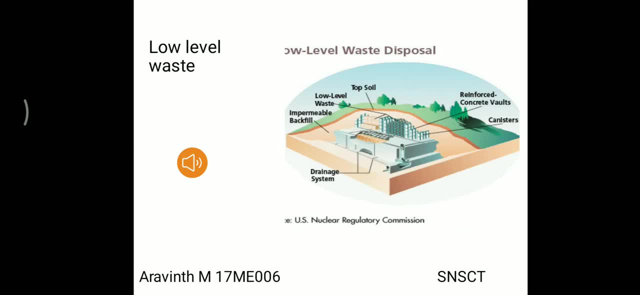 technically proven. The international consequence is that geological disposal is the best observed. The Types of Radioactive Waste: In this slide we are going to see about low level waste, that is, LLW, short form. LLW has a radioactive content not exceeding 4 GPa per tonne Of alpha activity or 12-beta-gamma activity. LLW does not require shielding during. 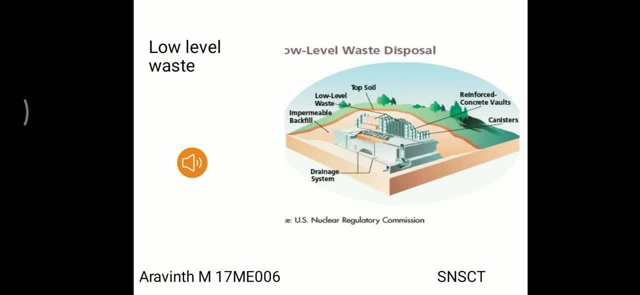 handling or transport. This is suitable for disposal in nearly surface facilities. LLW is generated from hospitals. The Dutch luxury company is selected by the annual risk-debit rate of $30,000 per station. The LLW is also the best for the industrial use. 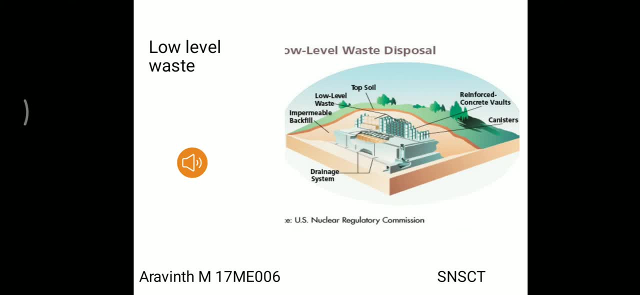 Large-scale electronic computers, building-structures, accelerators and solar panels are used as the source of radioactivity in the industries such as the nuclear field cycles. It composes paper records, Napoleon oil filters, etc. It contains small amounts of mostly short lived radioactivity To reduce its volume. LLW is often compacted or inclined before disposal. LLW comprises some 90% of the volume, but also 1% of radioactivity of all radioactive waste. The data Tribe, The new slide, is used to assess the high level of radioactive waste and the current activity of LLW. 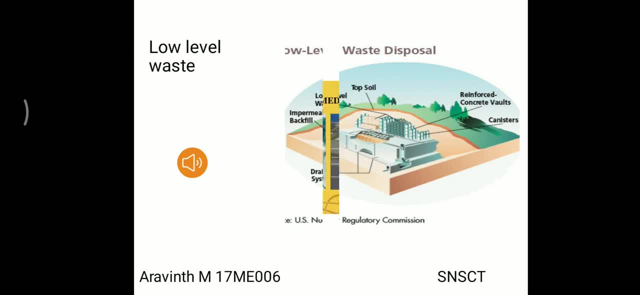 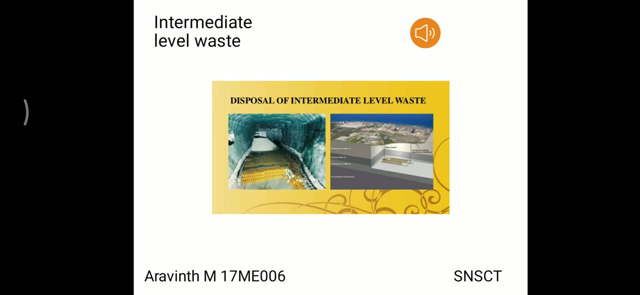 intermediate level waste. In this slide we are going to see about intermediate level waste, that is, ILW. ILW is more reactive than LLW, but the heat generator is not sufficient to be taken into account in design or selections of storage and disposal facilities. 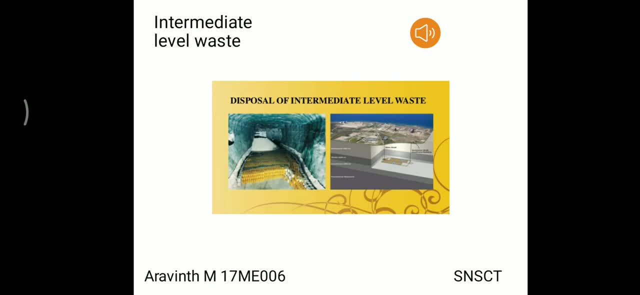 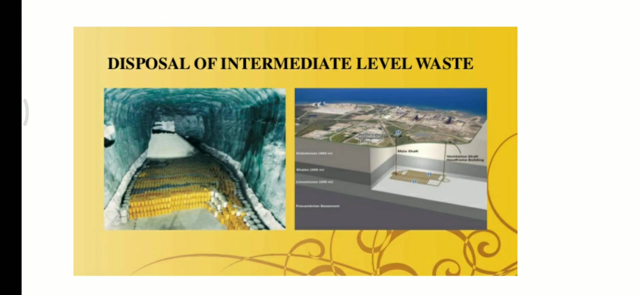 Due to its higher level of radioactivity, ILW requires some shielding. where notifying is LLW does not require any shielding. ILW typically comprises resin, chemical sludge and metal fuel cladding, as well as contaminated materials from reactor decomposing smaller items and non any solid may be solidified. 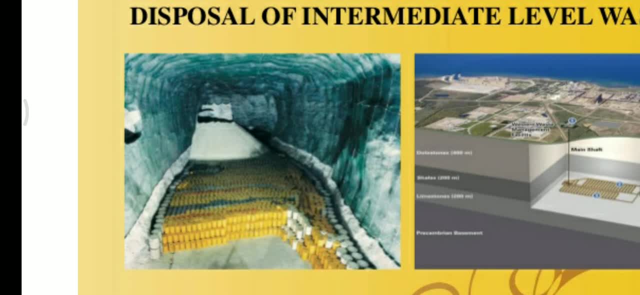 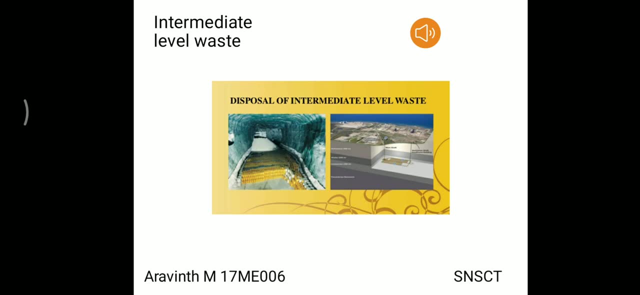 in concrete for disposal. It takes up some space. In this slide we are going to see about intermediate level waste, that is ILW. ILW is more reactive than LLW- This Negative Enterprise. In this slide we are going to see about high level waste, that is HLW. 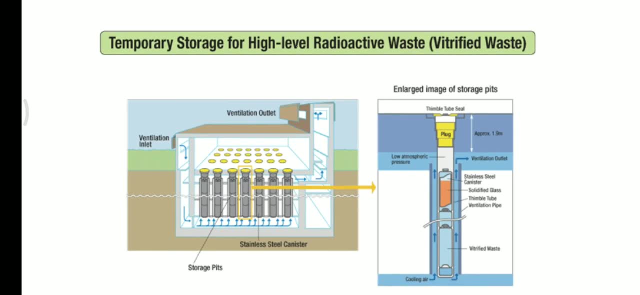 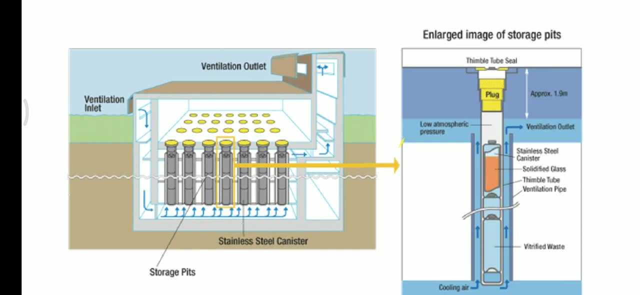 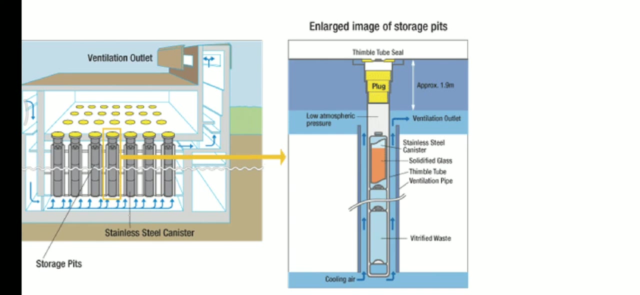 HLW is sufficiently radioactive for it's decay heat to increase it temperature and the temperature of it's при freezer surrounding significantly. As a result, HLW requires cooling and sealing. HLW arises from the burning of uranium fuel in a nuclear reactor. HLW contains 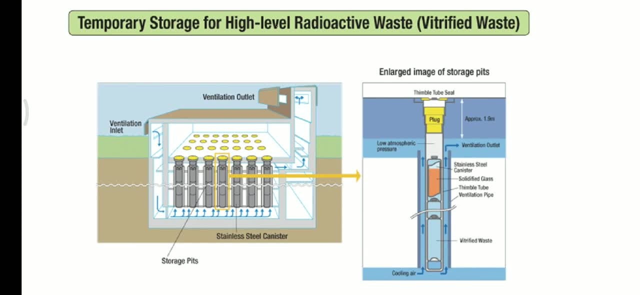 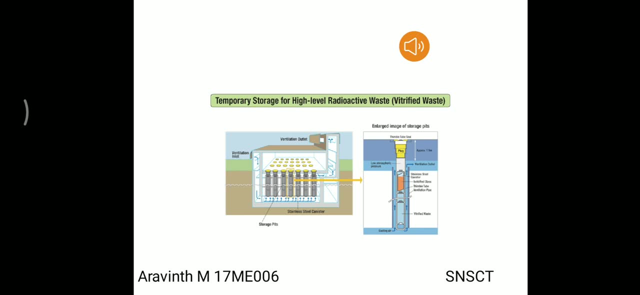 the fission products and transuranic elements generated in the reactor core. HLW accounts for just 3% of volume but 95% of total reactivity of product waste. They are two distinct kinds of HLW: Used fuel that has been. 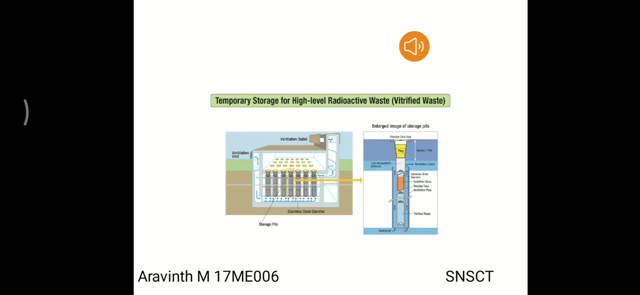 designated as waste, Separate waste from reprocessing of fuel cell. HLW has both long-lived and short-lived components, Depending on the length of the time it takes for the reactivity of the particular radionuclides to decrease to levels that are designed for that. 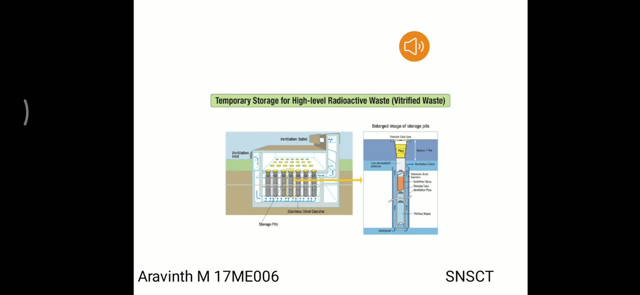 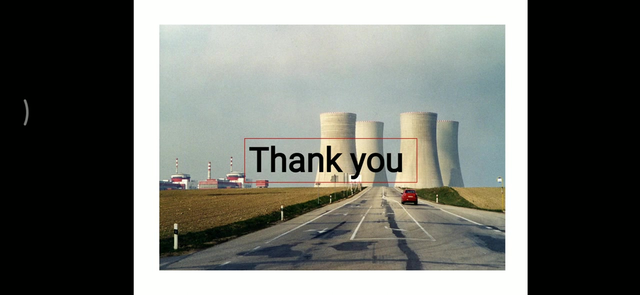 HLW is considered non-hazardous for people and surrounding environment. Generally, short-lived fission product can be separated from long-lived actinides. This disconnection becomes important in management and disposal of HLW. For more information, visit wwwhlwcom.